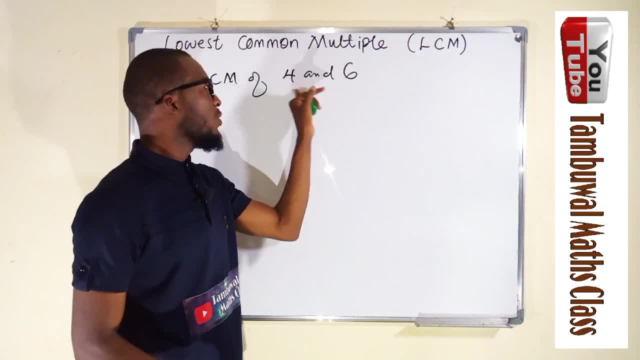 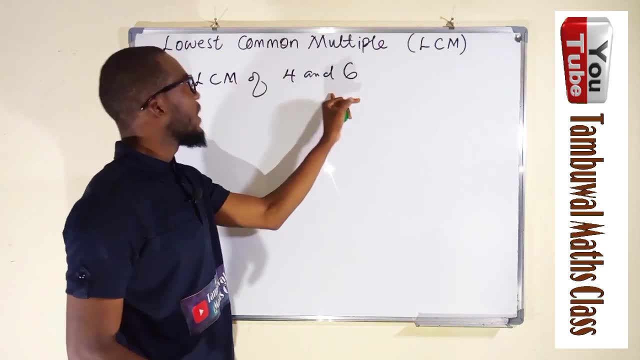 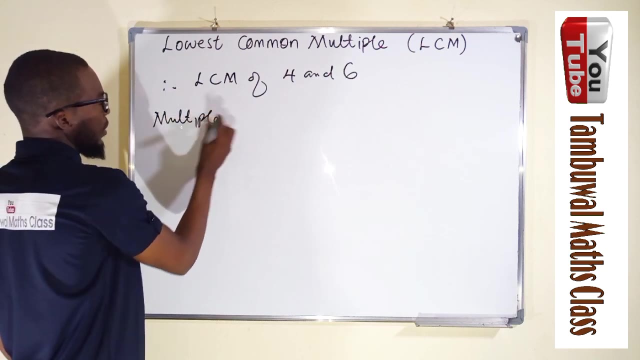 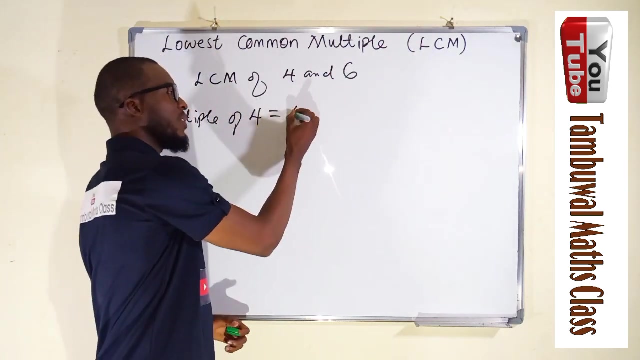 Now we want to find the LCM of four and six. Therefore, we are going to list out the multiples of four and six, Then take the common ones, then choose the least one Multiple of four from multiplication table. Four times one is four. Four times two is eight. Four times three is four. 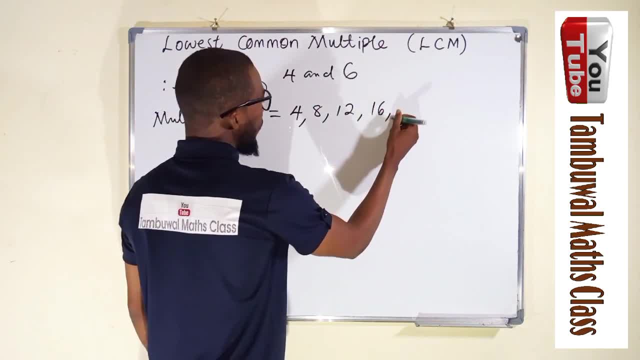 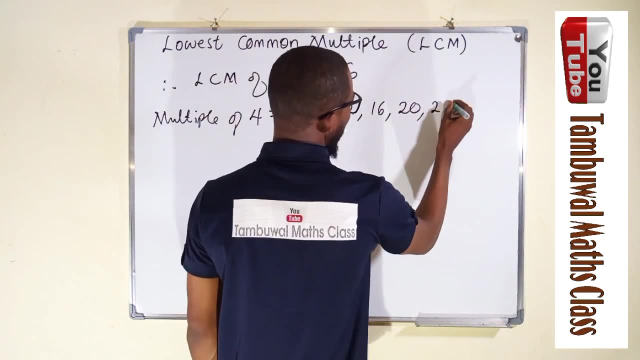 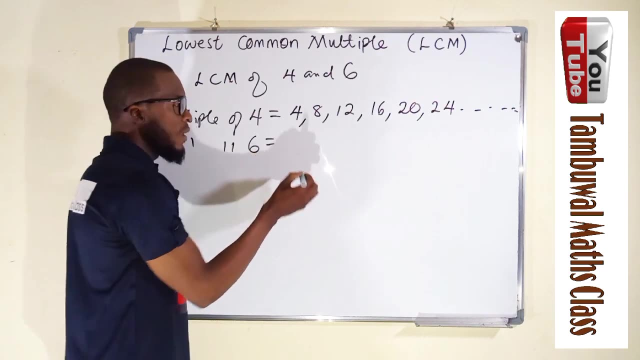 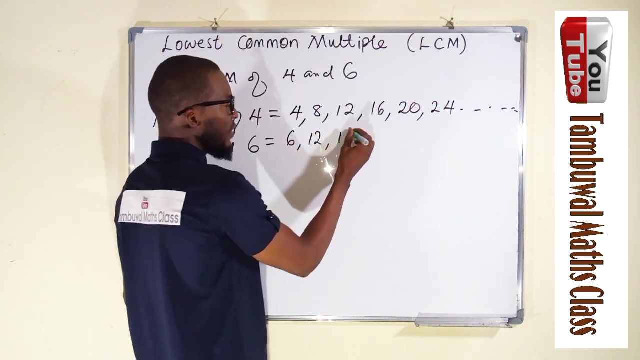 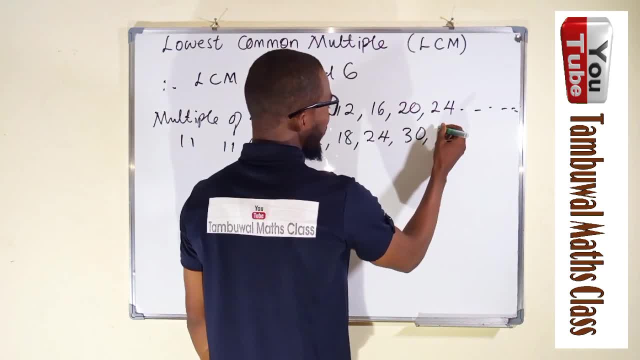 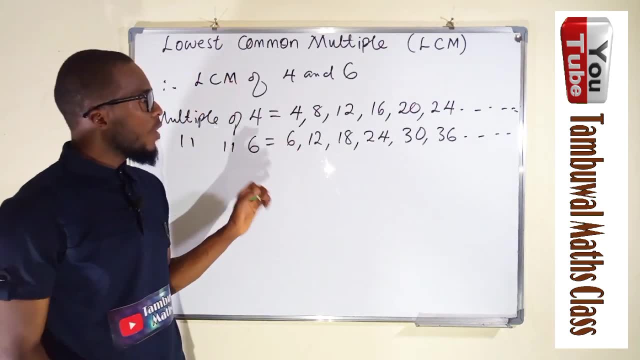 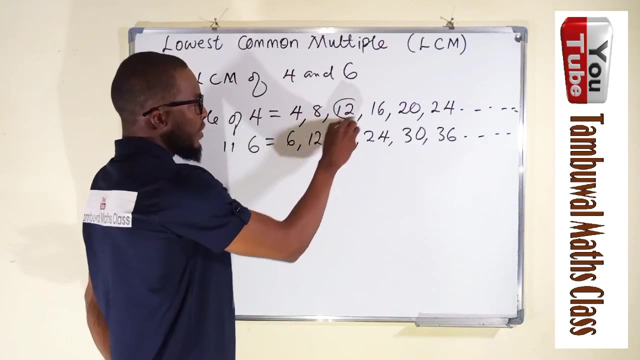 6 times 5 is 30.. 6 times 6 is 36.. We can stop here. So these are some of the multiples of 4 and 6.. Now we want to choose the common ones that appear here and here. From here you can see 12 here, We have 12 here, We have 24 here and we. equally have 24 here. Therefore the common multiples between 4 and 6 are 12 and 24.. But we are interested in knowing the least or the lowest, And lowest here is 12.. Therefore we say the LCM of 4 and 6 is 12.. 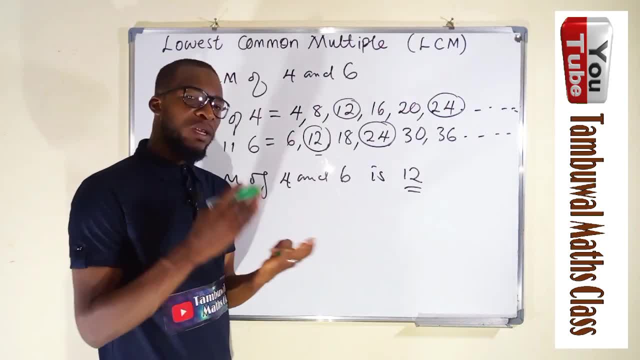 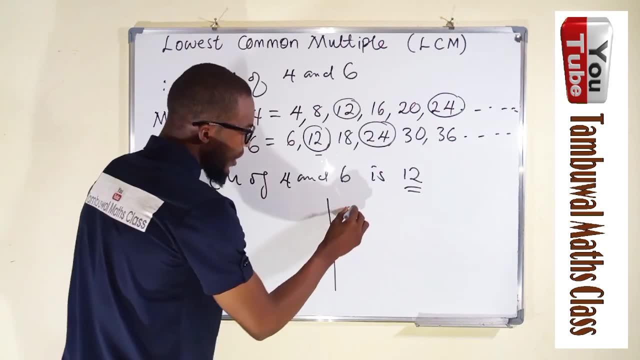 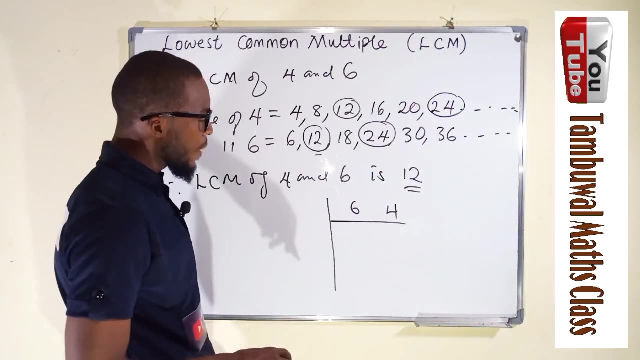 But the simplest way to do that is to perform a successive division of these numbers using prime numbers. We have 6.. We have 4.. You can start with either one. We are going to divide them through by some of the prime numbers, The least prime number. 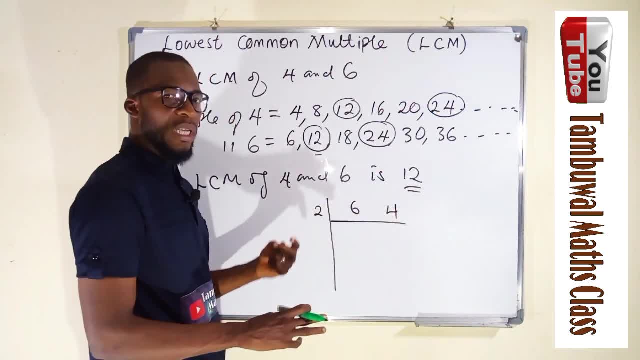 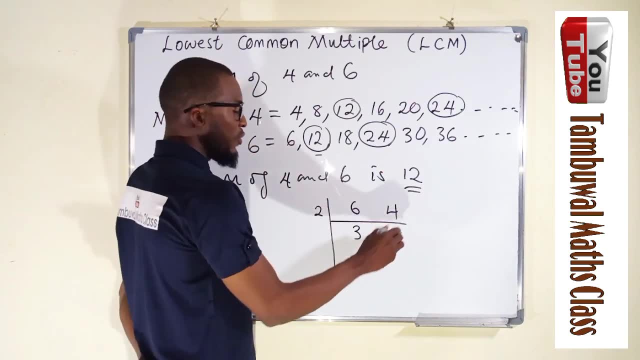 is 2.. You have to check whether 2 can go into these numbers. If it can't, you take the next prime number, which is 3.. 2 can go into 6 three times. 2 can go into 4 two times. 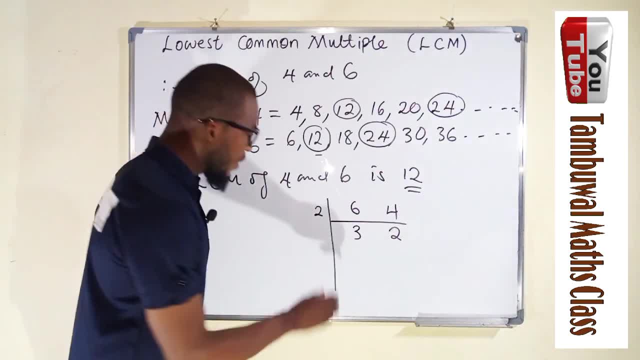 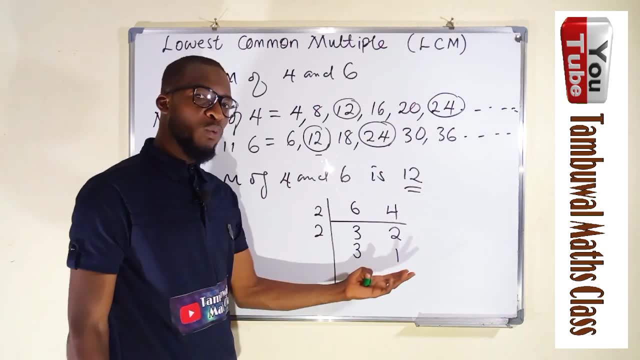 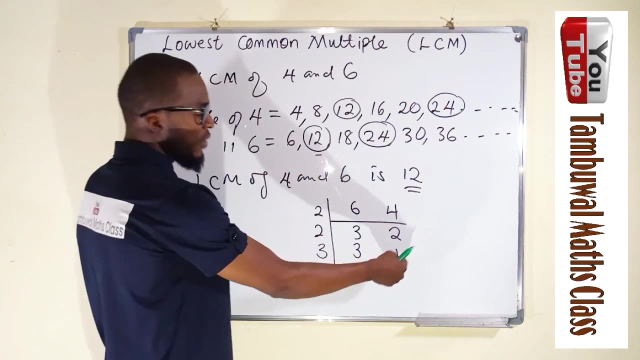 2 cannot go into 3, but it can go into 2.. Therefore, we have to try 2 again. You skip this. It can go into 2 one time. Once you reach 1, you stop. The only prime number that can go into 3 is 3.. So we use 3.. This one is already 1.. Therefore, the LCM of 4 and 6 equal to you. multiply them all: true, 2 multiplied by 2, multiplied by 3.. 2 times 2 is 4.. Then, 4 times 3 is equal to 12, as required. Therefore, 12 is the LCM of 4 and 6.. Why is this method very important? is in case. 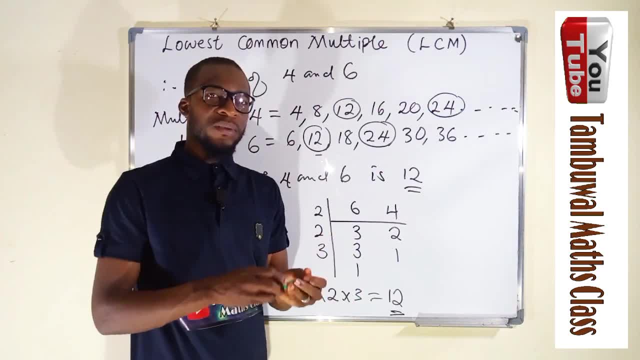 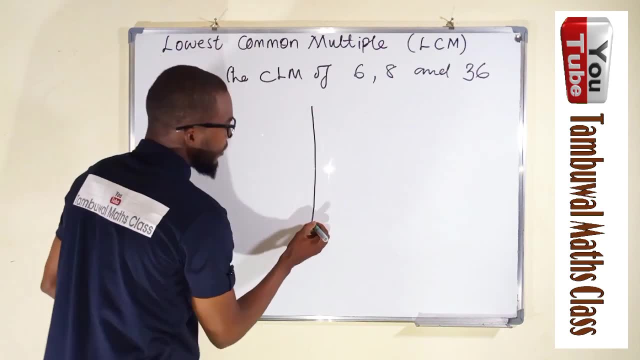 of larger numbers. Now let us try some numbers. Now we want to find the LCM of 6,, 8, and 36.. We are going to perform a successive division of these numbers- 6,, 8, and 36- using prime numbers. 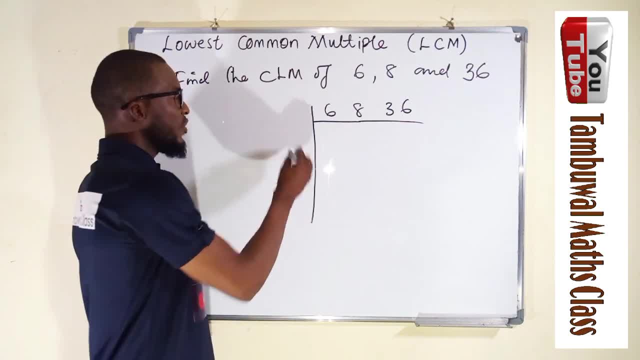 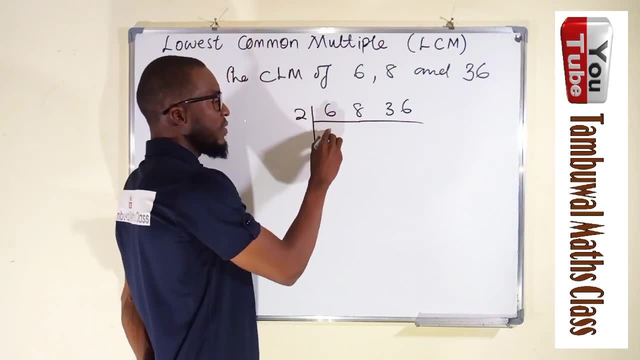 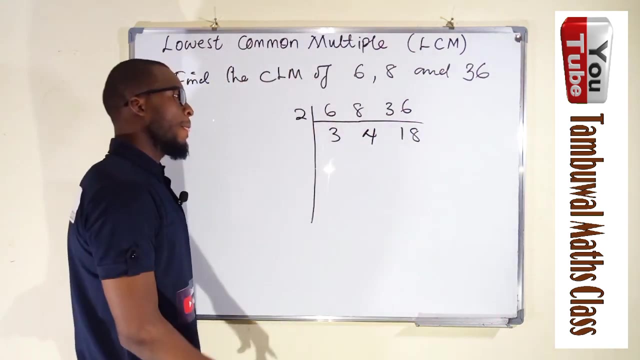 All these numbers are even numbers, so we can try the least prime number, which is 2, because 2 can go into any even number. 2 into 6 is 3.. 2 into 8 is 4.. 2 into 36 is 18 times. We still have some. 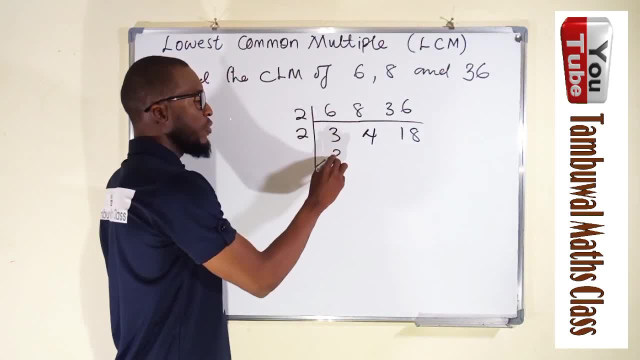 even numbers. We are going to try the least prime number, which is 2.. 2 into 6 is 3.. 2 into 8 is 4.. 2 into 9 is 9.. We have 2.. It cannot go here. You drop this down. 2 can go into 4, 2 times 2 can go. 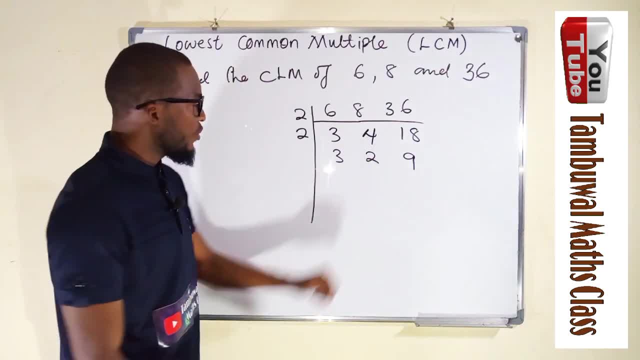 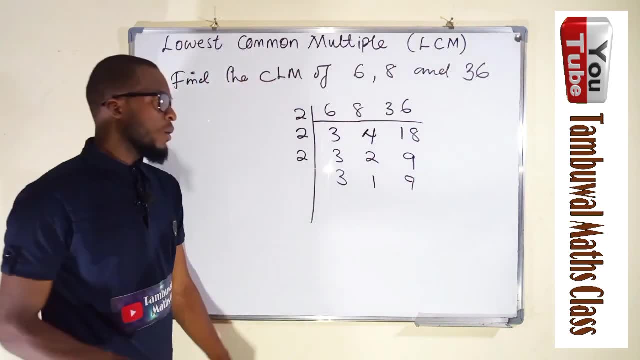 into 8 and 9 times. We still have another even number, 2.. You drop this down. It can go into 2 one time. You drop this down, 2 cannot longer go into any of this. You try the next prime number. 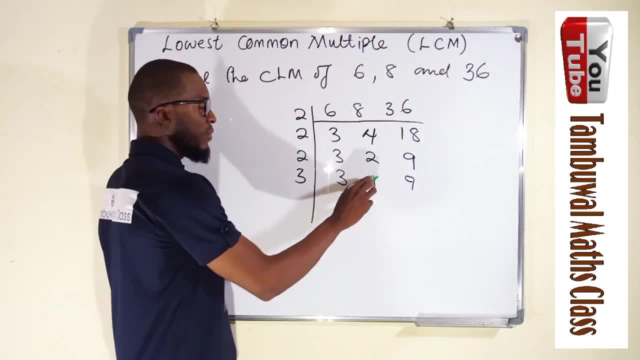 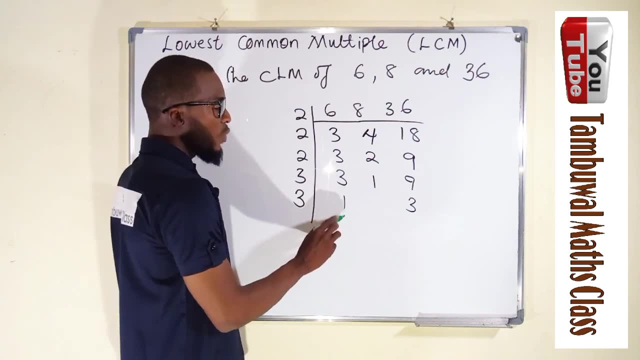 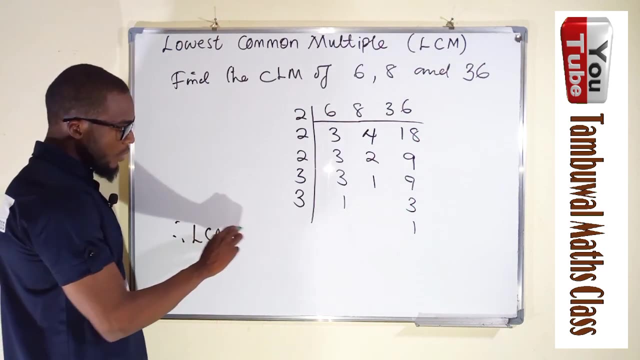 which is 3.. 3 can go here one time. This one is already 1.. It can go here 3 times. Still, we have 3.. This is already 1.. We have 1.. It can go here 1 time. Therefore, the LCM of 6,, 8, and 36 will be. 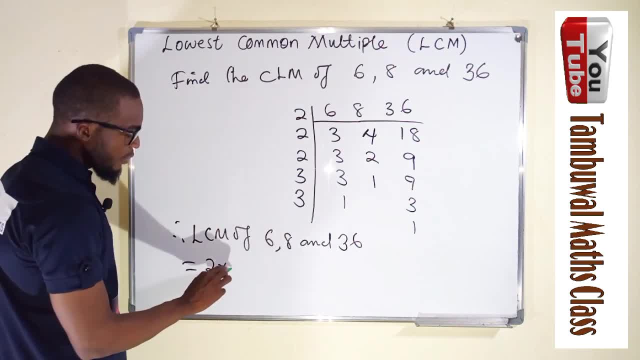 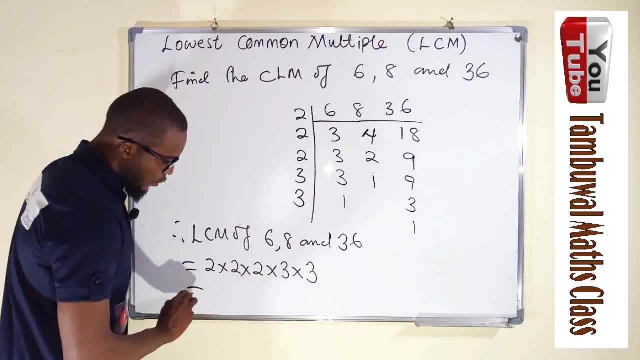 equal to you. multiply all these numbers: 2, multiply by 2, multiply by 2, multiply by 3, multiply by 3.. This is equal to: 2 times 2 is 4.. 4 times 2 is 8.. 8 times 3 is 4.. 4 times 3 is 8.. 4 times 3 is 8.. 24.. Then 24 times 3 is 72.. Therefore, the LCM of 6,, 8, and 36 is 72.. It is the only smallest number which these three numbers can simultaneously go into without remainder. So this is very important while simplifying fractions or while trying to eliminate fractions. 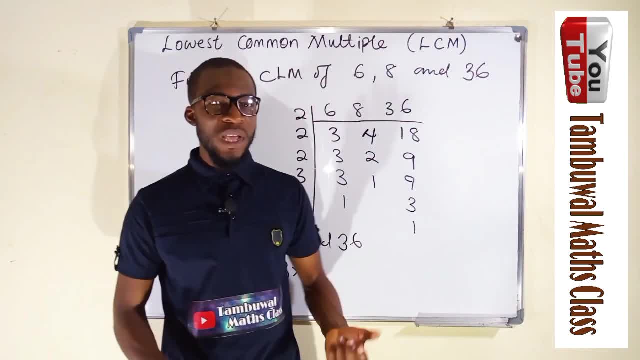 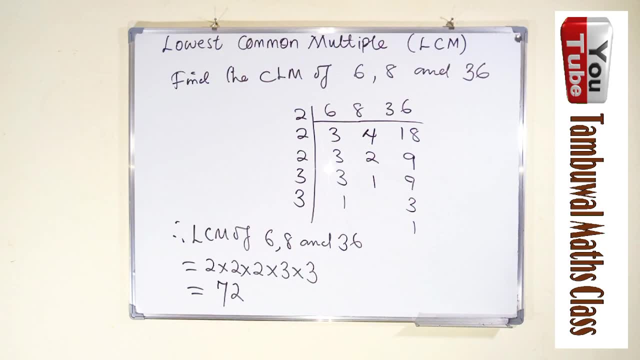 in a given equation. Thank you for watching. Do have a nice day. Thank you for watching. Do have a nice day.